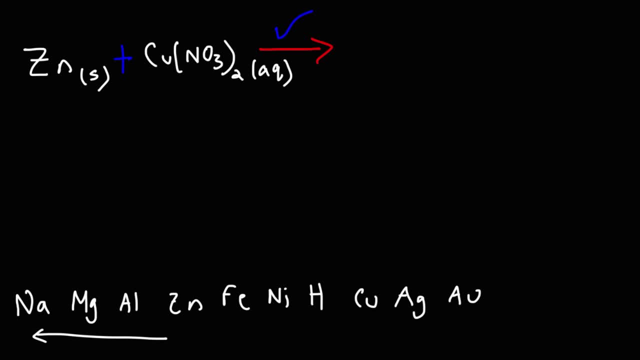 And the answer is yes, This reaction will proceed. as written. Now we need to determine the products of this chemical reaction. We know copper is going to be displaced out of the solution. Right now it's in the aqueous phase, which means that it's dissolving water. 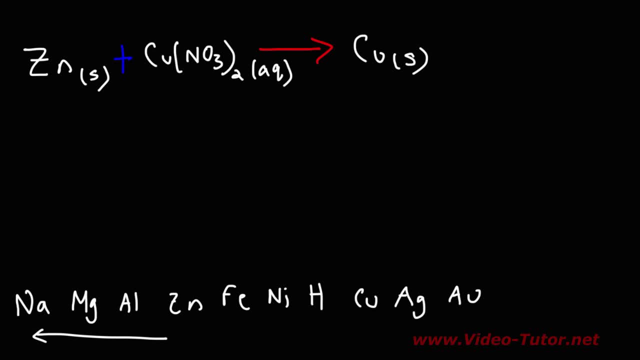 But it's going to pick up some electrons from zinc metal and it's going to precipitate as copper metal out of the solution. The zinc is going to be displaced out of the solution. Zinc is going to pair up as it's going to pair up with nitrate. 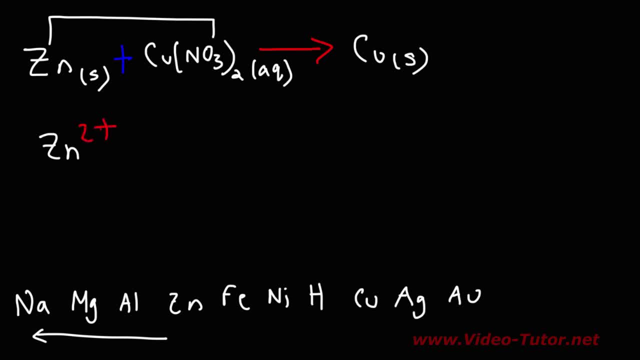 The zinc is going to lose two electrons, turning into the zinc 2 plus ion. Nitrate is a polyatomic ion with a minus 1 charge. So in order for these to neutralize each other, we need one zinc ion and two nitrate ions. 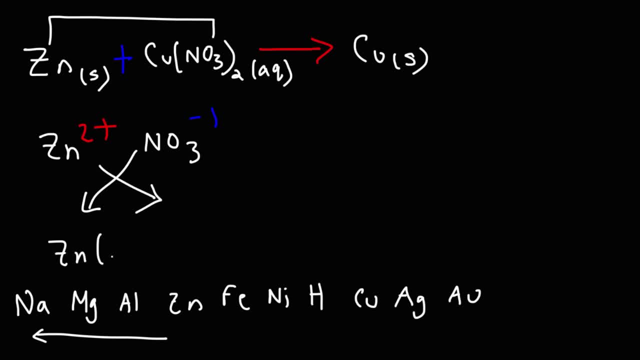 So the chemical formula of zinc nitrate is going to be ZnNO3 2. And nitrates are always soluble in water, so this is going to be in the aqueous phase. So that's how we can predict the chemical- I mean the products- of this particular single replacement reaction. 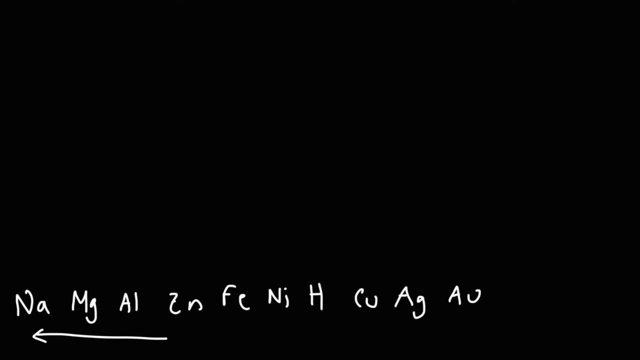 Now let's move on to our next example. In the next example, we're going to mix iron metal, so this is in a solid state, with hydrochloric acid. So this is 8.5.. This is aqueous. 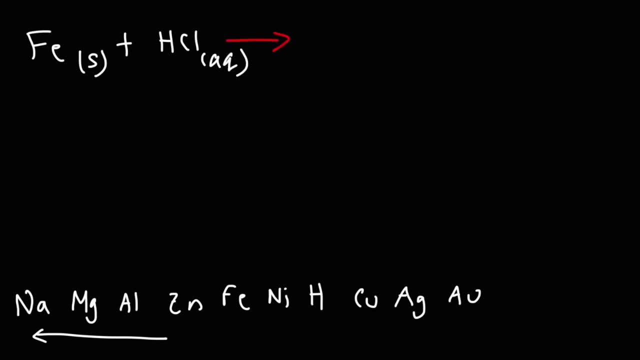 Go ahead and predict the products of this single replacement reaction. Note that iron is to the right of hydrogen, so this is going to work. Fe is going to pair up with Cl. Iron metal is going to give up two valence electrons, turning into the Fe2 plus ion. 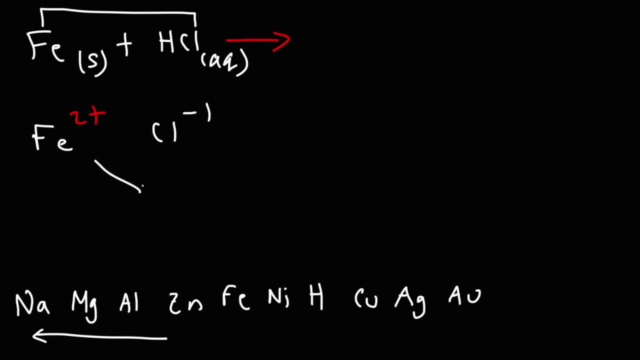 Cl has a minus 1 charge. So when you pair these two together, you're going to get the chemical formula Fe1Cl2.. Or for short you could just say FeCl2.. Now, chlorides are generally soluble, except with silver, lead and mercury. 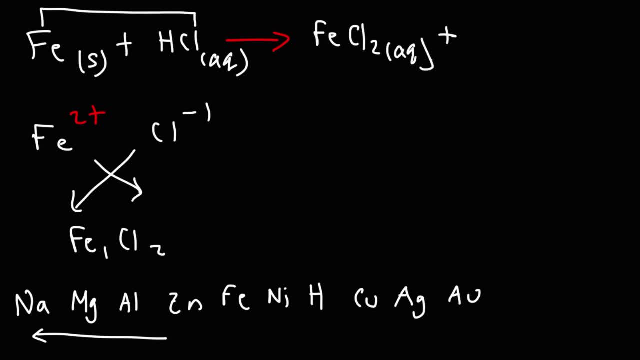 So this is going to be in the aqueous phase. It's important to know the solubility rules, especially when dealing with reactions such as this. So when iron metal gives up its electrons- for those of you who want to know what's happening, 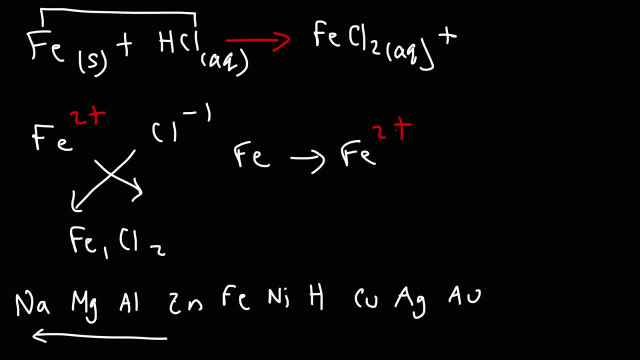 iron metal is going to turn into Fe2 plus And it's going to give away two electrons. This is an oxidative process. Whenever a substance gives away electrons, it's oxidation. The hydrogen ions will pick up those two electrons and they will turn into hydrogen gas. 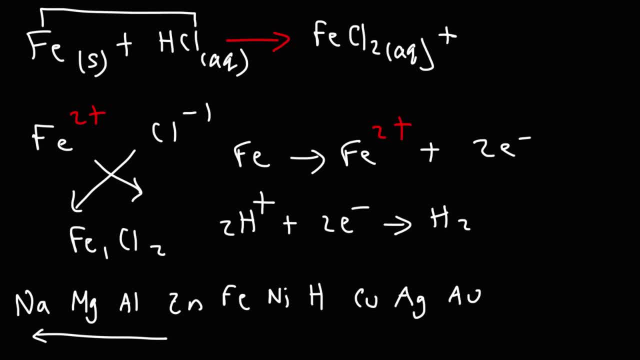 This is reduction. Anytime something acquires electrons, it's being reduced, So hydrogen gas will evolve from the solution Now the only thing we need to do now is balance the chemical equation. We have two hydrogen atoms, Atoms on the right side. 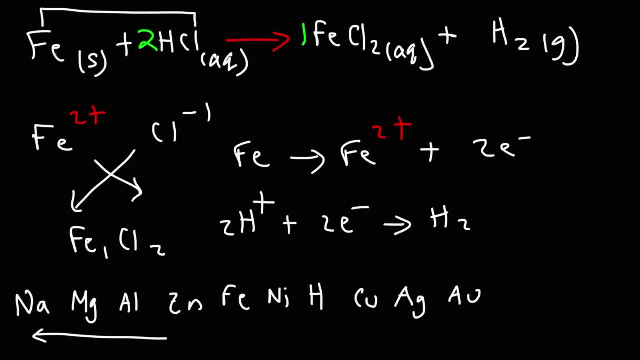 So we need to put a 2 in front of HCl, And after that everything else is balanced. So that's it for this example problem. Let's move on to the next one. Let's react aluminum metal with aqueous nickel sulfate. 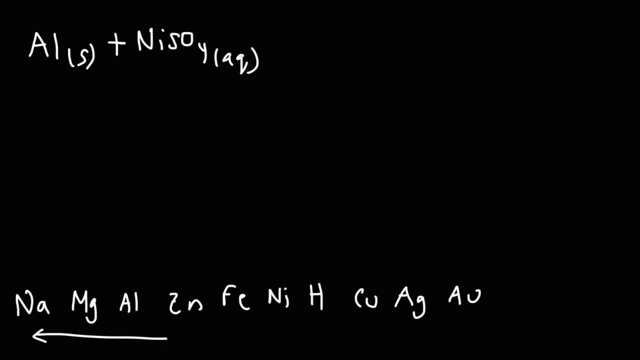 Go ahead and predict the chemical. I said that wrong. Go ahead and predict the chemical. Go ahead and predict the products of this chemical reaction. So aluminum is going to pair up with sulfate When aluminum gives up its 3 valence electrons. 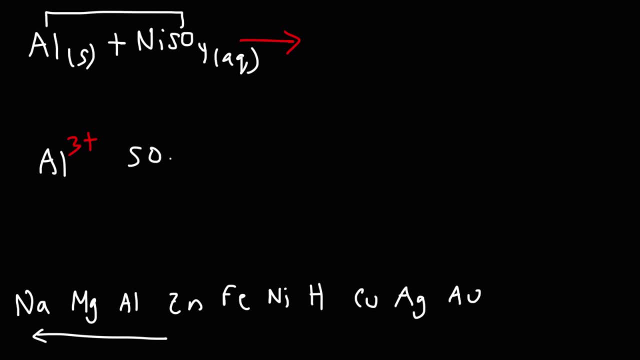 it's going to turn into. the aluminum 3 plus cation Sulfate is just one of those polyatomic ions you have to commit to memory if you haven't done so already, So using that crisscross method that we've been using. 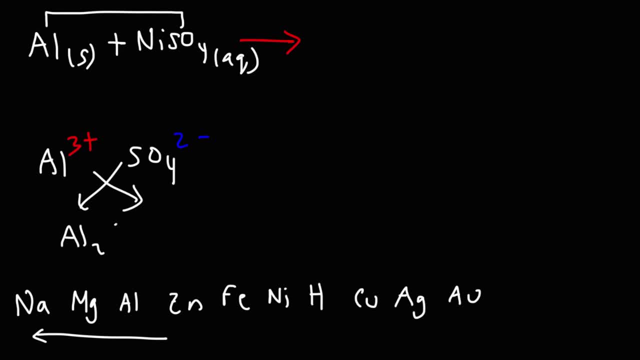 when these two get together, they will generate a chemical formula, Al2SO43.. And the reason why we're doing this is because we know that it works that way. it's due to charge balance. We need two aluminum ions to get a total charge of 6 plus. 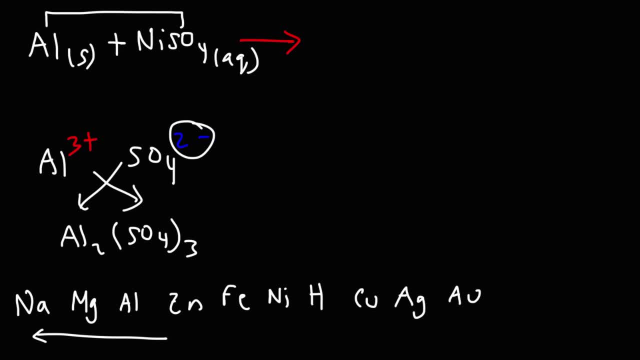 We need three sulfate ions to get a total charge of 6 minus, 6 plus and 6 minus. they're the same- just opposite- in sign. So the charges have to be equal and they have to balance each other out. So that's why we get that particular chemical formula. 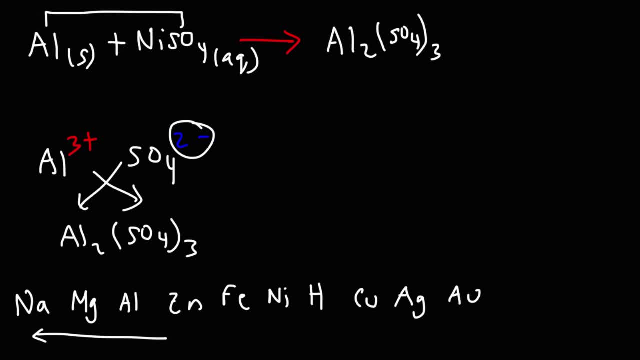 And sulfates are generally soluble, with the exception of certain group 2 elements like calcium, barium and even lead. But with aluminum, sulfates are soluble. So this is going to be an aqueous phase And nickel is going to precipitate out of the solution. 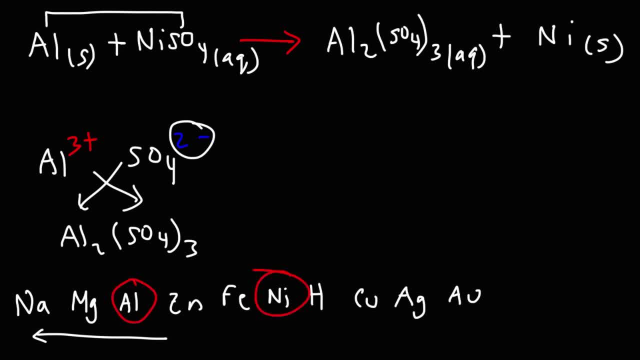 Looking at the activity series, aluminum is much more active than nickel, So these are the products of this single replacement reaction. But now let's go ahead and balance the equation. So we have two aluminum ions on the right side. We need to put a 2 in front of Al. 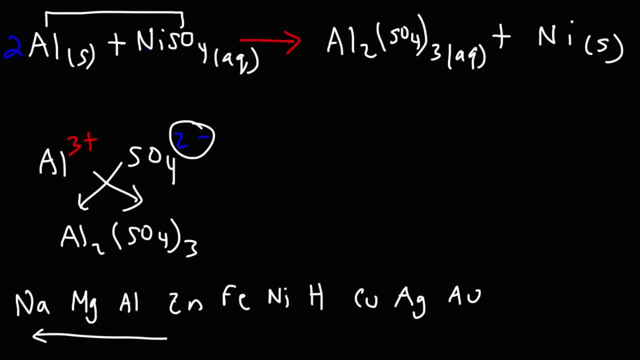 We have three sulfate ions on the right side, So we need three in front of NiSO4.. We can put a 1 here. Now we have three nickel ions on the left. We need a 3 in front of nickel on the right. 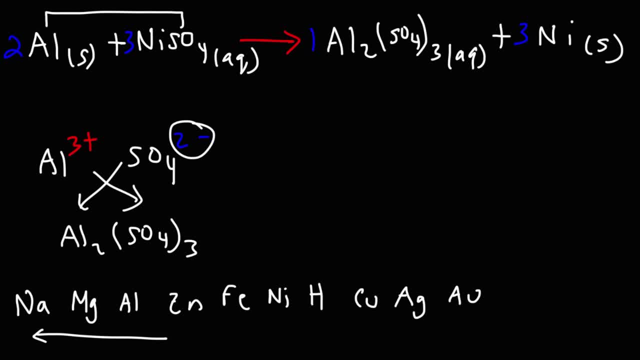 So now our single replacement reaction is balanced. Here's another example for you. So let's say we bubble in hydrogen gas Into a solution of copper sulfate- What's going to be the products of this reaction? So this reaction will also work. 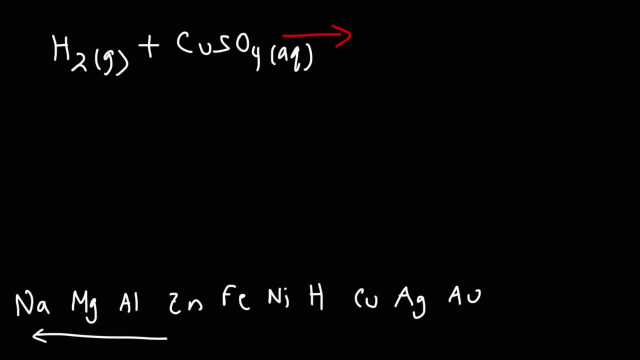 Because hydrogen is more active than copper. So for those of you who want to know what hydrogen is going to do is it's going to turn into the H plus ion, releasing two electrons, The copper 2 plus ion in copper sulfate. it's going to pick up those two electrons and be reduced to copper metal. so 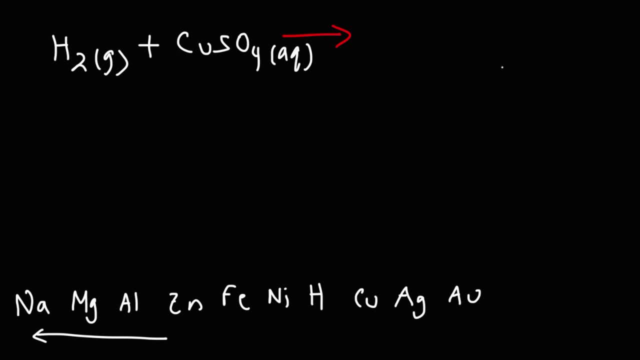 hydrogen is going to displace copper out of the solution. thus we're going to get solid copper and then, if we pair up H plus and the sulfate ion, we're going to get H2SO4, or sulfuric acid for short, and sulfuric acid is soluble in water. now we don't need to balance the chemical equation. 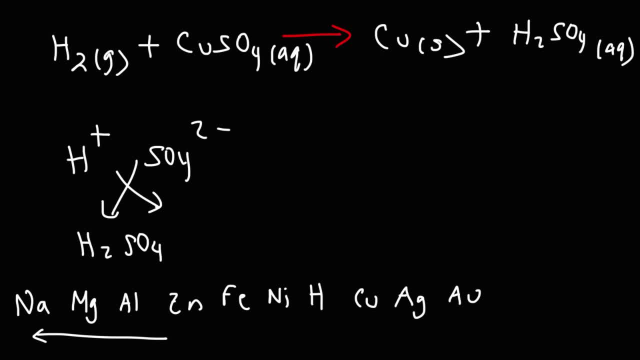 because it's already balanced, and this is it. so this is the. these are the products of this particular single replacement reaction. we have copper, metal and sulfuric acid. now let's consider another example: liquid bromine is mixed with a solution of potassium iodide. what's going to be the products? 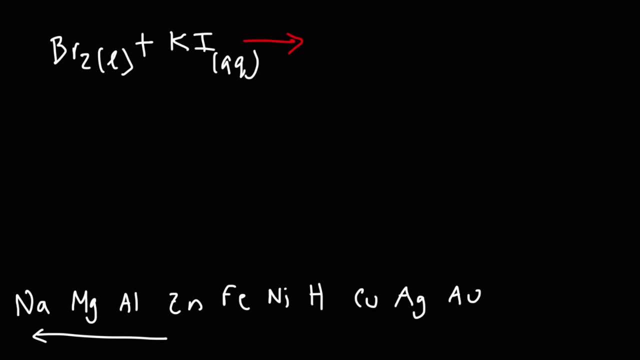 of this reaction. now we also need to consider the activity series of the halogens. fluorine is much more active than chlorine, which is much more active than bromine, and that's more active than iodine, so fluorine can displace chlorine out of a solution in this. 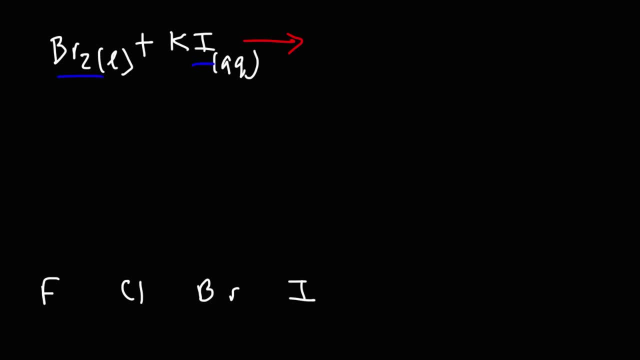 example, bromine is strong enough to displace iodide out of the solution. but just so you know what's happening here, bromine is acting as an oxidizing agent. non-metals: they like to acquire electrons, so iodide is going to give away two of its electrons, turning into one of its electrons. 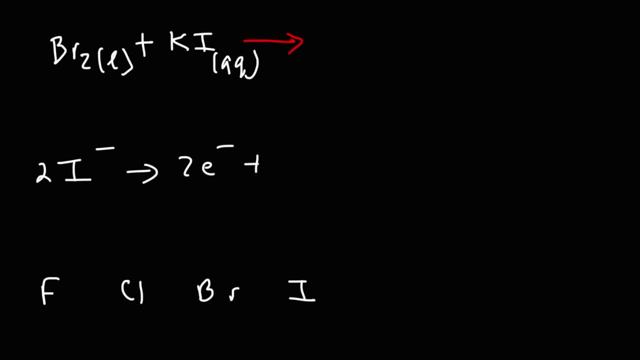 so iodide is going to give away two of its electrons, turning into one of its electrons. so with theOkay. so I think that's probably enough, put just 있게er. so what we need to figure out is what this is actually is. I think we're going to start with one solution at them and starting with iodine, and then we're just going to 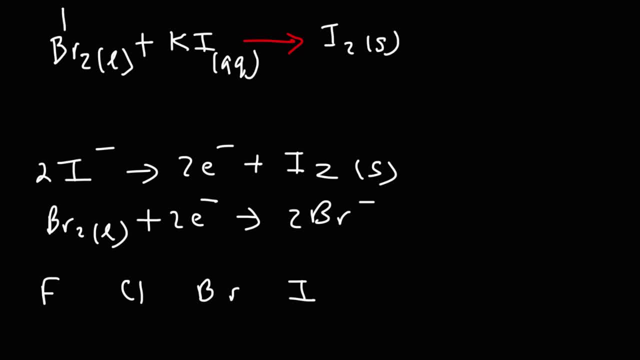 hook up the salt br and played up two super ez pair up with K. So potassium naturally has a charge of plus one. Bromine, as an ion, will have a charge of minus one. So because the charges are equal in magnitude, you can simply write them in. 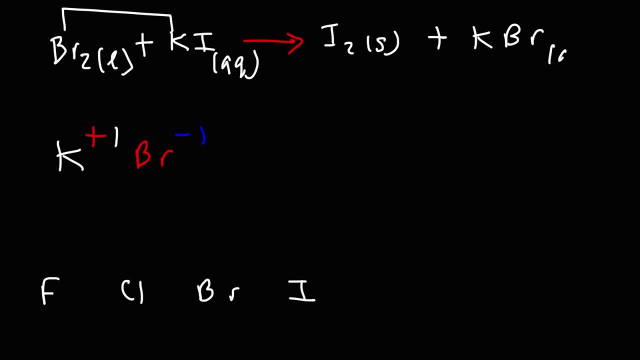 a one-to-one ratio. So we're going to get KBr, and that's soluble in water. The last thing we need to do here is balance the chemical equation. All we need to do is put a two in front of Ki and KBr. 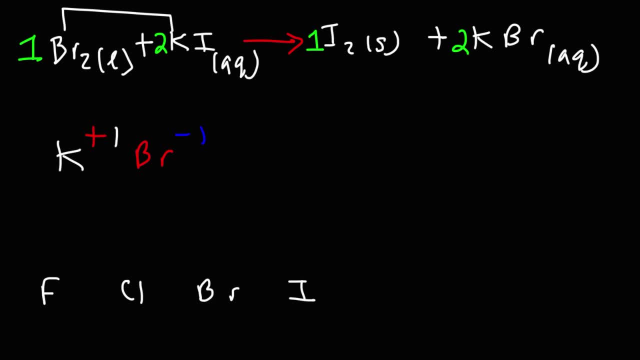 and then it's going to be balanced. So that's it for this video. Now you know how to not only predict the products of a single replacement reaction. you also know how to determine if the reaction will proceed and how to balance it as well. Thanks for watching.